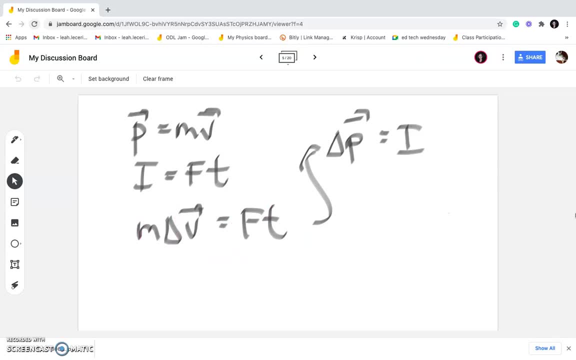 moreappropriate and it adds up to a certain number of variables and then we can use the it looks more useful when it comes to problem solving right so basically this is a change in momentum and another way of writing that would be mass times Delta V right we've explained that before and then impulse is force times time so basically these two are just different forms of the same thing now going forward let's look at the other possible variations of that okay now example suppose you have a impulse momentum problem which gives you the mass the change in the velocity or Delta V as well as the force and then the required to find is time okay so how does the final equation look like in this kind of problem so I think the best thing to do is to start with how the impulse momentum theorem looks like conceptually which is like this change in momentum equals impulse right okay and then let's look at the other given in the problem we have mass change in velocity force and time if you look closely none of these variables are directly shown in this particular problem or directly given so 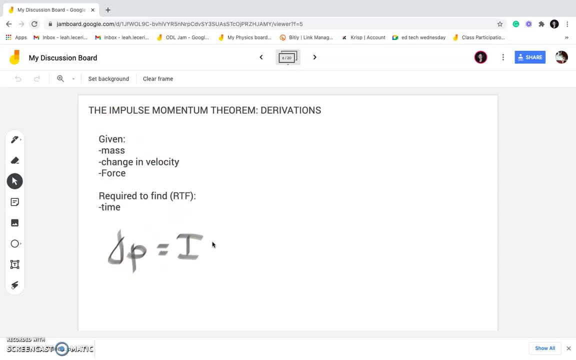 we would rather chunk them down into their what I would call like their 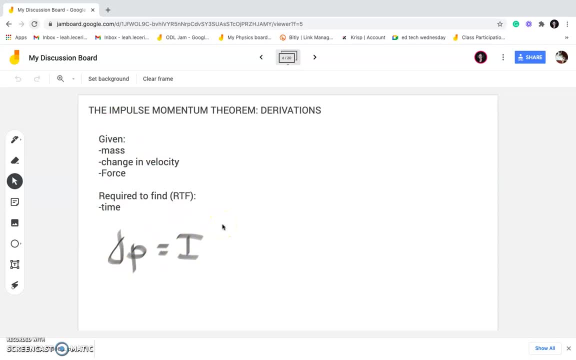 components or their equivalents right so Delta P would be M times Delta V right because momentum is a change in momentum 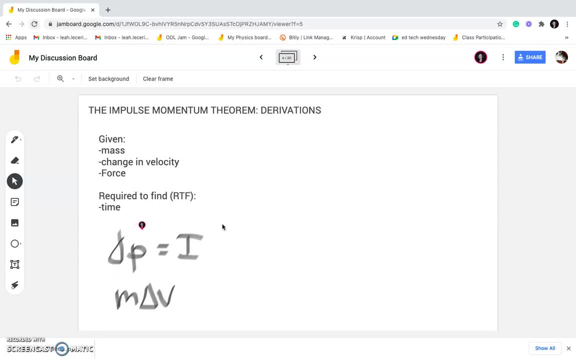 rather or Delta P is equivalent to M Delta V right okay and then for I or impulse we're gonna make it force times time so nothing bloody it's just that impulse is equivalent to force times time it's that simple okay and this is 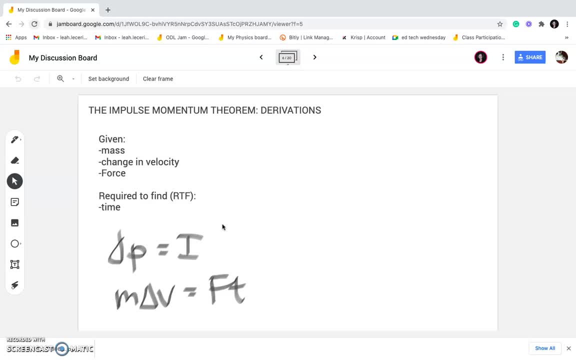 better because it actually matches the given variables in the problem like we have mass right there and then the Delta V is also known in the problem you also have force in the problem and then they're required to find is time which is also here in our equation so this is a better way of writing the final working equation instead of this one although my point in teaching this kind of thing is 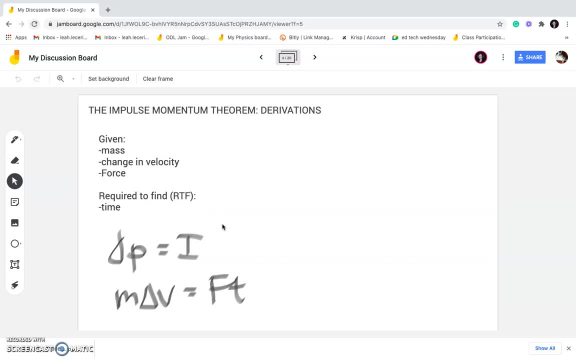 for you to see that this simple equation can actually take different forms depending on the problem and it's better to sometimes start with this one because when when students tend to start with this one which is more important than the other one because when students tend to start with this one which is more detailed they tend to get lost when the problem looks slightly different and not 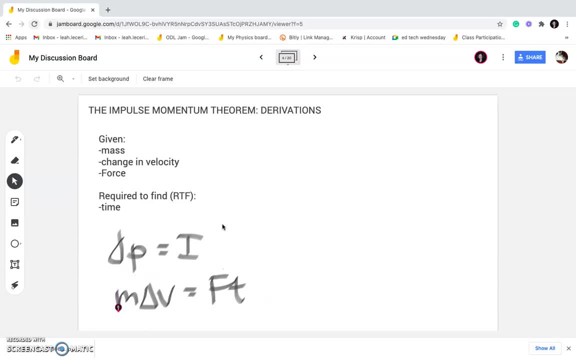 exactly fitting with this equation so I think that the best thing to do is always remember this major equation and from there you can derive all other different forms that are all just similar okay so lastly we're going to divide both sides by F why is that so it's simply because the required to find is time therefore we have to isolate time so in this case we can cancel force already on the right side so we're gonna have M Delta V over F equals time so this is our final working equation you can flip it horizontally so that time is on the left side but they're actually just the same going forward another sample situation is you have initial velocity mass force and time as the given and the required to find is final velocity so once again the impulse momentum theorem says that the change in momentum or P is equivalent to the impulse imparted on the system okay but do we retain these variables as they are let's see in the given we have mass and final initial velocity right so what we can do instead is write the change in momentum as M times final minus 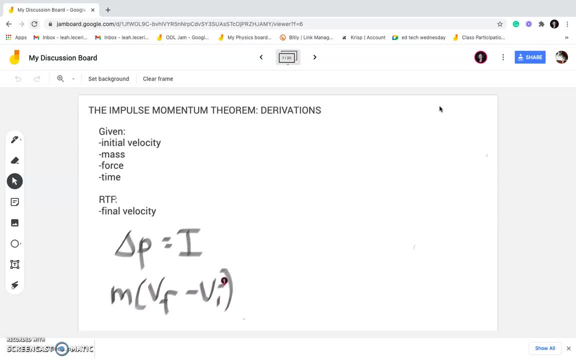 initial velocity okay now if you find this confusing it's not really that confusing it's just that we're used to seeing change in momentum to be like this okay M Delta V right that's what we've been used to seeing so far change in momentum is equivalent to M Delta V however if you look at the given you don't have Delta V it's not directly giving you the change in velocity you have the initial and the final states of the velocity and they recall the fact that change in velocity is actually equal to final minus initial velocity so in other words this expression M Delta V can also be written as M times V sub F minus V sub i in an enclosed parentheses so instead of Delta V we have V sub F minus V sub i okay now going forward the so i think i would write something that can divide this yeah there okay so going forward we will write uh um equals um four times time easy uh it's because impulse is forcing sign right okay and we don't want to write impulse alone because we don't have it in the problem but we have force and time anyway so we would rather write impulse as the product of force and time to fit the given in the problem that's how it works okay now the the rtf is final velocity so we need to isolate this one the final velocity okay how do you do that um since this is enclosed in a parenthesis 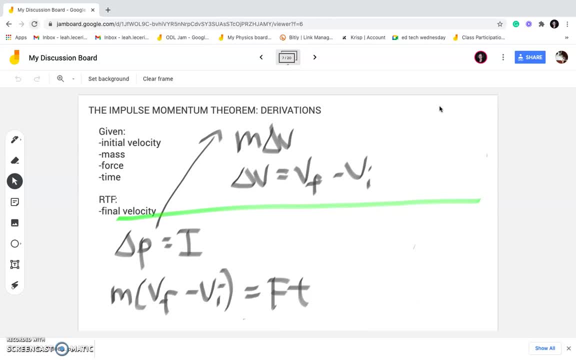 what we can easily get rid of is m right so we will divide both sides of equation by m and this can be cancelled on the left so we're gonna have v sub f minus v sub i equals f p over m okay now what happens next since we want to isolate final velocity in the problem since it's the rtf right or we're simply going to transpose v sub i to the right so that v sub f will be fully isolated and it will look like wait i'll just erase this one for more space okay so the final working equation would then be v sub f equals f t over m plus v sub i so nothing bloody what we did is just we transpose v sub i on the right so 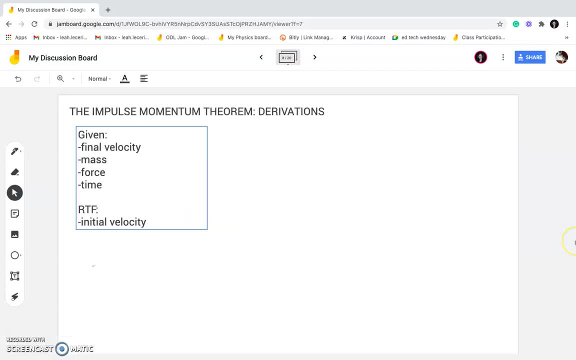 the negative sign becomes positive for the next example we have a very similar um problem just like the one in the previous example except that the initial velocity is now the rdf so earlier 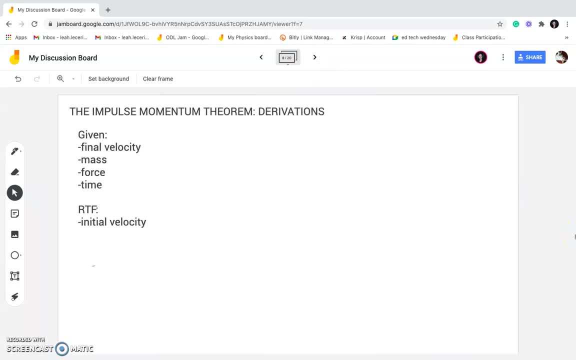 final velocity was the rdf so same thing we know the fact that the change in momentum is equal to and change in momentum or delta p could be m delta v and then impulse would be force times time now once again we have delta v or change in velocity in the equation but in the problem what we got is final initial velocity for the rdf okay so that will become m times v sub f minus v sub i equals force times time okay so basically we replace delta v with final velocity minus minus initial velocity because these 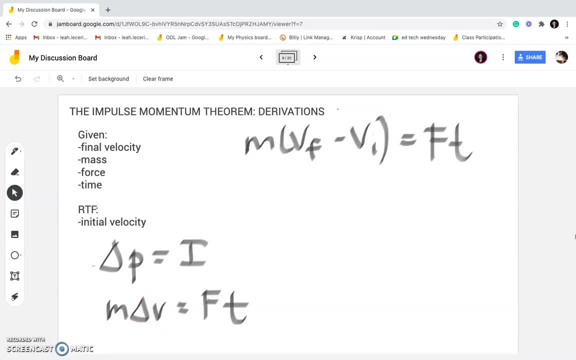 two are equivalent quantities okay change in velocity is v sub f minus v sub i 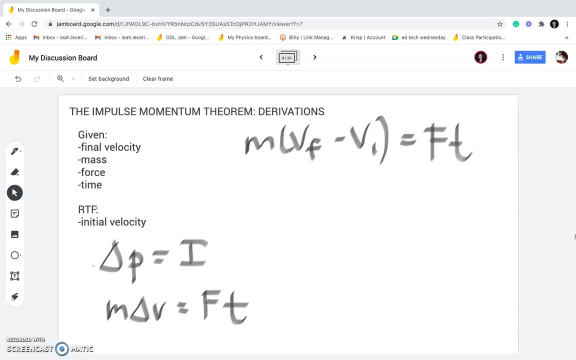 okay going forward um we will divide both sides by m just like last time so this will become vf minus vi equals fp over m and then for us to fully isolate the rtf which is the initial velocity 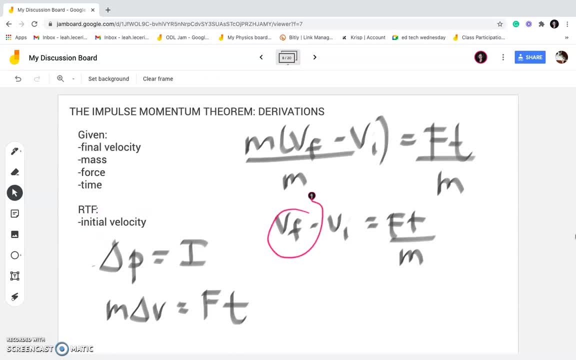 and we have to transpose v sub f to the right side of the equation so that will give us negative v sub i equals fp over m minus v sub f but of course we don't want the rtf to be negative so 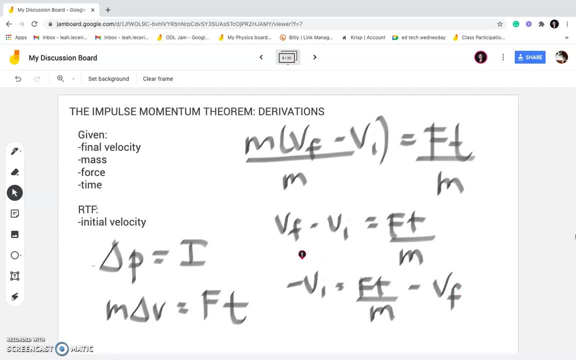 we will multiply both sides of the equation by negative one and this will give us b sub i equals negative fp over m plus v sub f 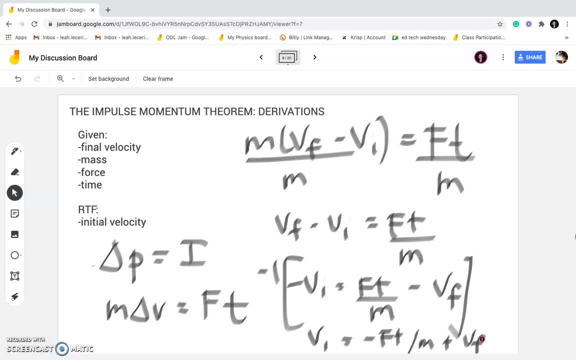 v sub f so the final working equation would be this one v sub i equals negative f t over m plus v sub f because we have to multiply both sides by negative one so this will become positive 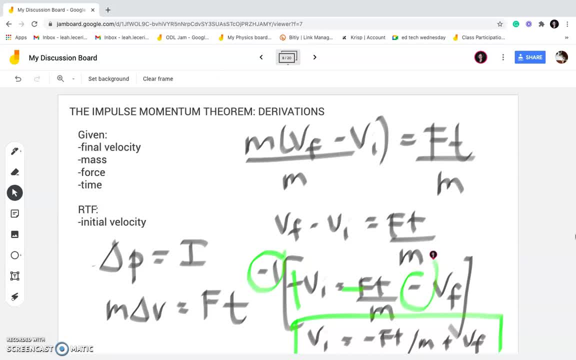 this will become negative then this one will become positive okay that's it okay going forward 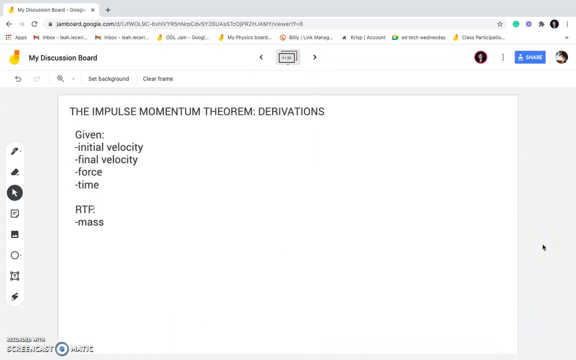 um one last example for this particular given we have initial velocity final velocity force time and then the required to find is mass so basically um once again the principle says that change in momentum a change in momentum is equal to impulse so we're going to replace delta p with 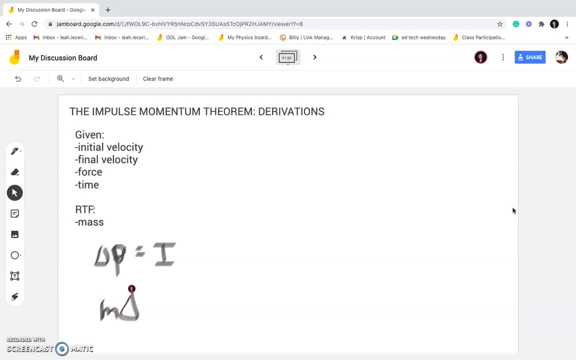 m delta v and then impulse would be better written as force times time 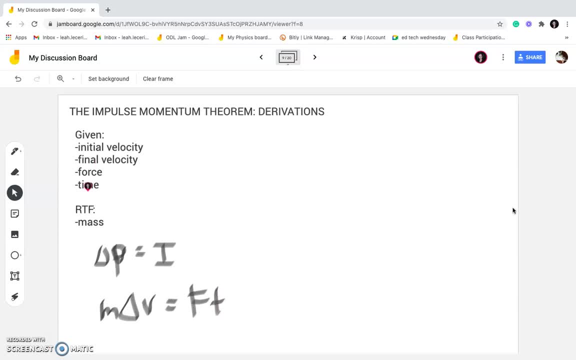 right because we have force and time in our given and then delta v must also be replaced with initial and final velocity because we don't have delta v right but we have the initial and the final values of the velocity so this will become m times v sub f minus v sub i equals force times time okay now since the rtf is mass we're going to divide both sides by v sub f minus v sub i for us to easily cancel all those expressions in the parentheses eventually isolating m it's just it's that simple okay so this will be cancelled out it will become one right because v sub f minus v sub i divided by v sub f minus v sub i is one so this will become m on the left side and for the right side you have f t over v sub f minus v sub i so our final working equation in this kind of scenario or situation would be this one that's it for this video if you have any questions please feel free to ask me in the comments below 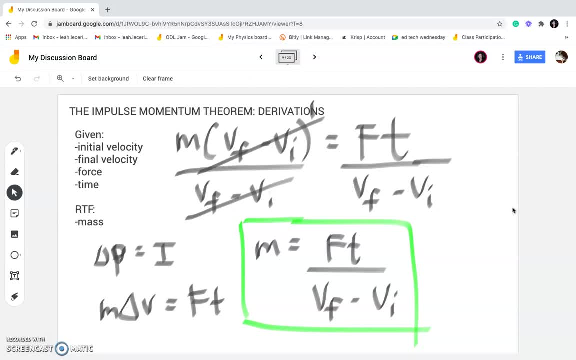 this video i hope that that uh was helpful for the for your preparation on the mathematical part of this lesson particularly the problem solving thank you so much have a great day